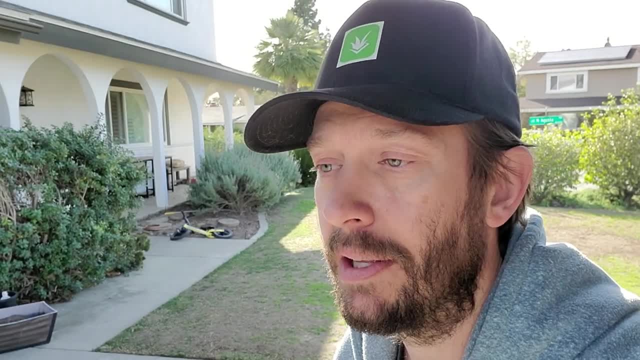 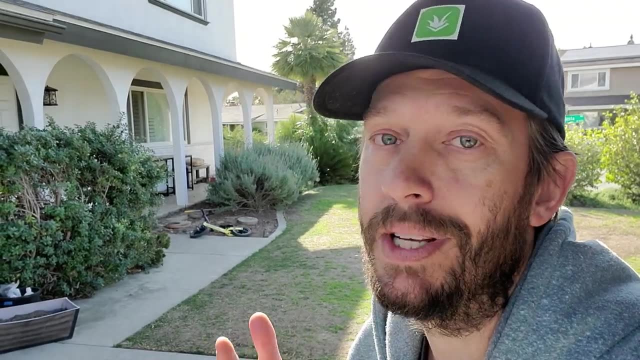 amounts of time and money to achieve a lawn like this. Now, I do spend more time than what I'm going to talk about in this video and I apply more products, but you don't need to. That's the thing You don't need to- The things that you actually need to make a lawn look fantastically. 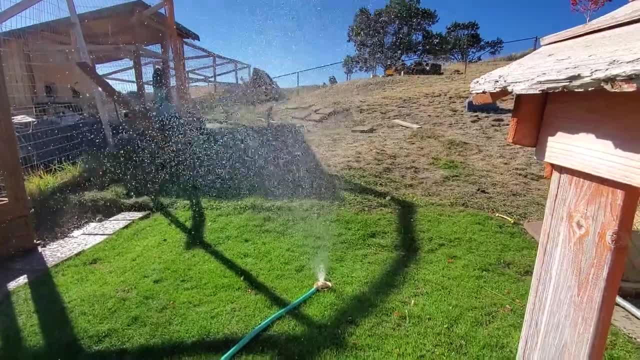 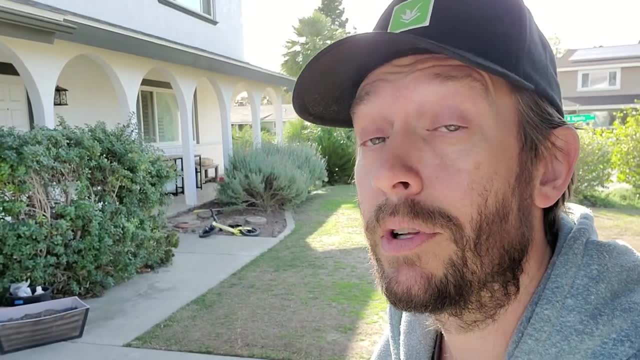 green and beautiful is sun, sunlight, water and nitrogen. That's it. That's really it. Nitrogen is the primary ingredient in lawn fertilizers. You can get fertilizers anywhere, Like I've seen them sold at my grocery store. You can get them. 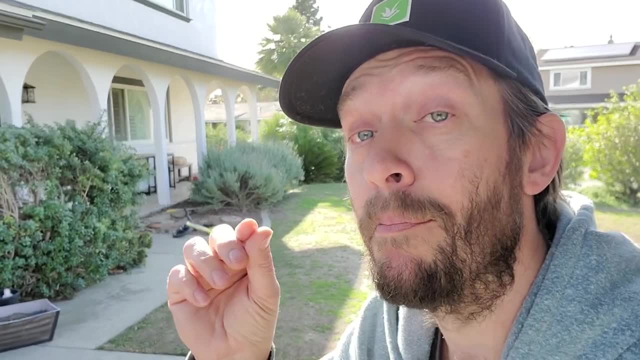 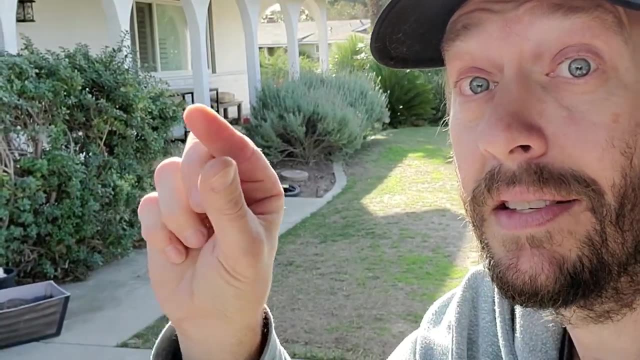 at big box stores. You can buy specialty stuff online. But the most important thing here is you want nitrogen. That's the first number on the NPK. N, That's nitrogen. Get yourself something high on nitrogen, like really high on nitrogen. 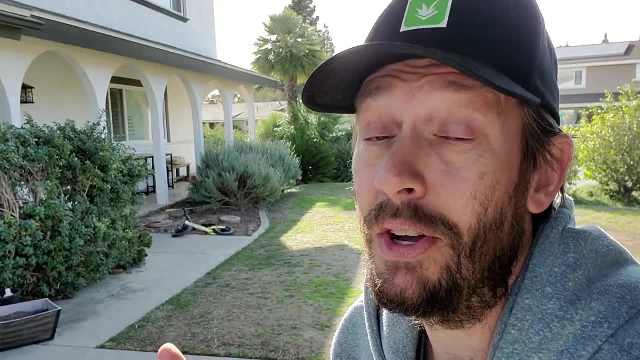 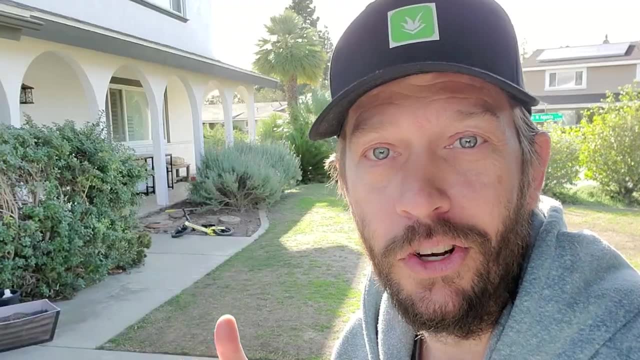 and then only apply it a few times throughout the year, And you'll be pretty good. If you apply it a lot of times throughout the year, you'll be even greener. Don't apply everything all at once, though, because then you'll burn your lawn Now, if you do take the time to actually put down a nitrogen, 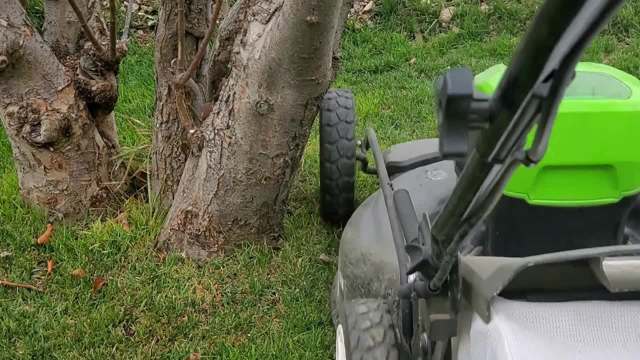 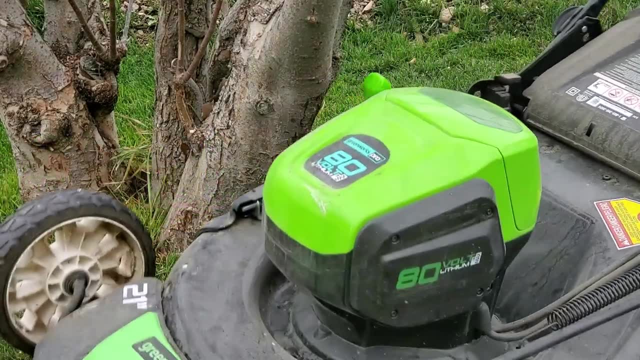 fertilizer on the lawn. you need to mow frequently throughout the course of the entire year. The video linked in the description below is all about the importance of mowing as often as you possibly can without going overboard. Please take a look at that. Water Mowing is very important. It's very 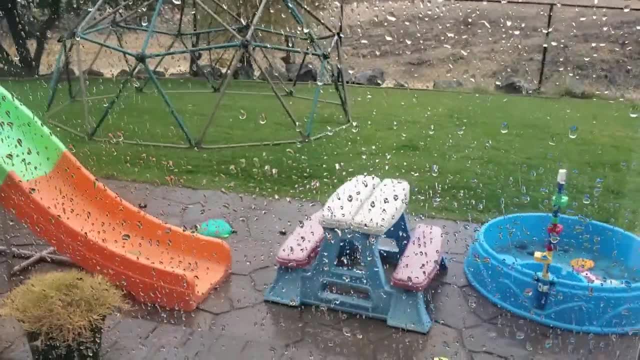 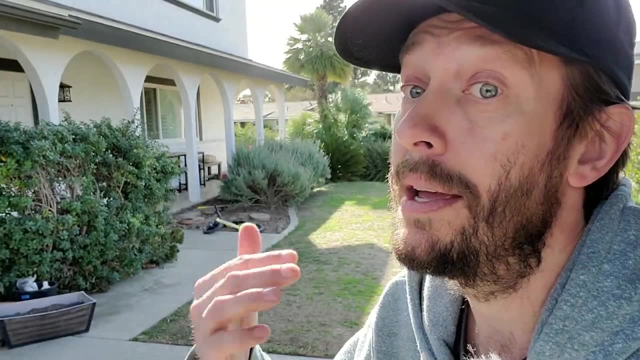 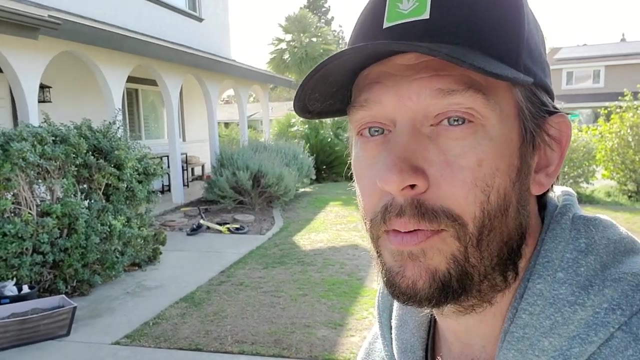 most people get water from the sky or from your irrigation lines, so your in-ground sprinklers or your above-ground sprinklers. Rule of thumb is: you only need one inch of water per week. I personally advise applying one inch of water one time per week instead of spreading it out. throughout the week. If you apply one time per week, then the upper layer of your soil, sometimes the upper few inches of your soil, will dry out, and that's fine, because the roots dig down deep underground. You'll always want them pushing deeper into the soil profile to look for. 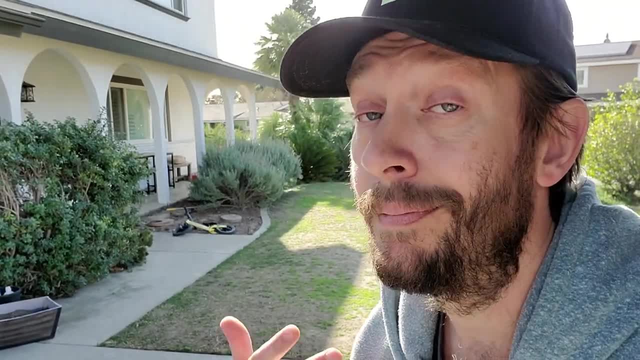 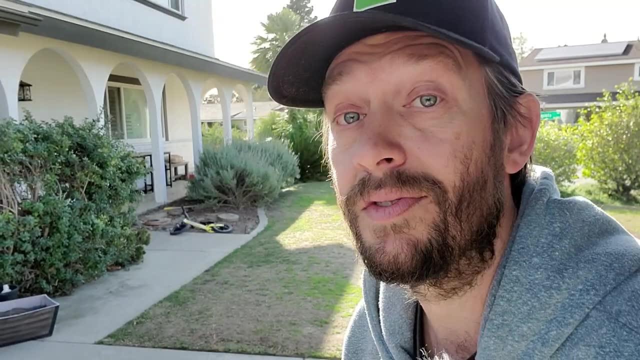 the deepest water source possible. If you're watering too often, that's never going to happen. Water infrequently and deeply In sunlight. you have, like, virtually no control over it. It's just the sun. Don't expect much of anything in the way of your lawn, regardless of temperatures between the months of October 31st, the months, the days of October 31st and approximately mid to late February. If you do live in a very cold climate or if you're growing a warm season grass further up north, then instead of late February, you're looking at more like late March.